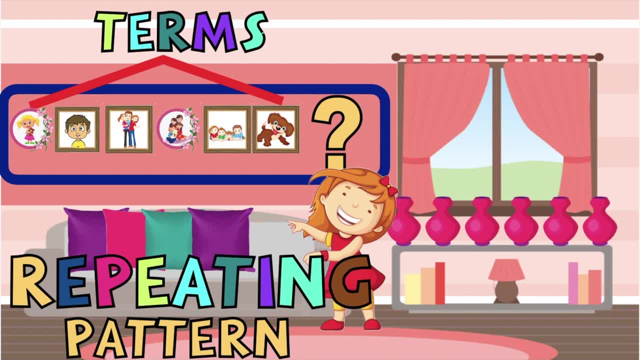 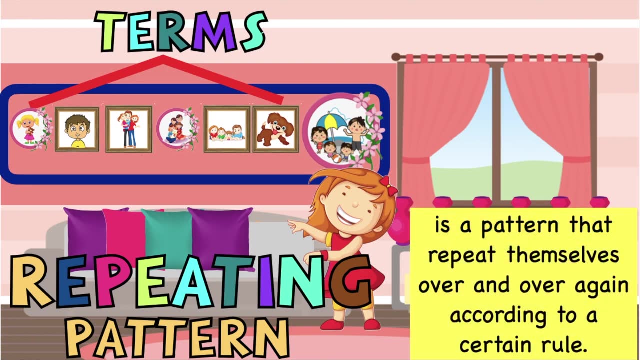 What do you think is the next term? That's correct, children. We're going to have a circle frame, Very good. So again, this is what we called a repeating pattern. When you say repeating pattern, it is a pattern that repeats themselves. 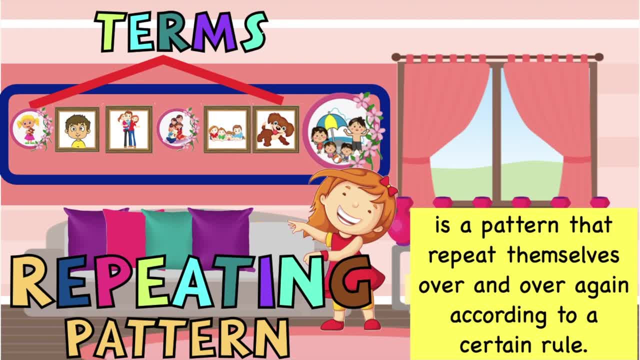 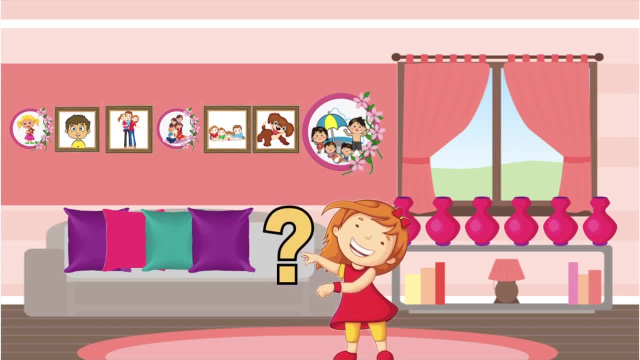 over and over again, according to a certain rule. How about, if we are going to arrange these pillows, What do you think will be the next pillow? That's correct, children. We're going to have a pink pillow. So this pattern is what we called a repeating pattern. 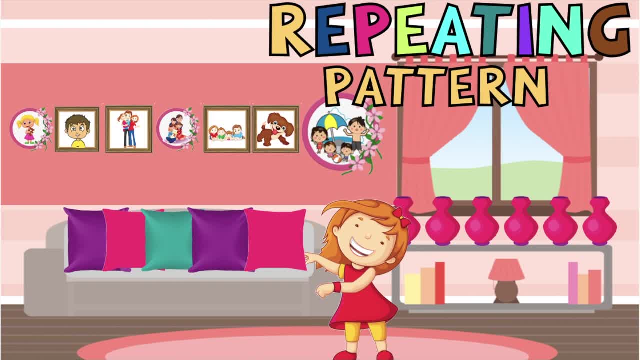 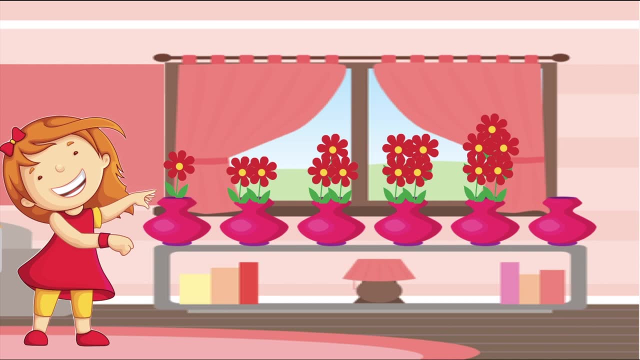 Always remember. repeating pattern is a pattern that repeat themselves over and over again according to a certain rule. So now, children, let's help Zarina arrange the vase. Zarina arranged sets of flowers in 6 vases. How many flowers should there be on the 6th vase? 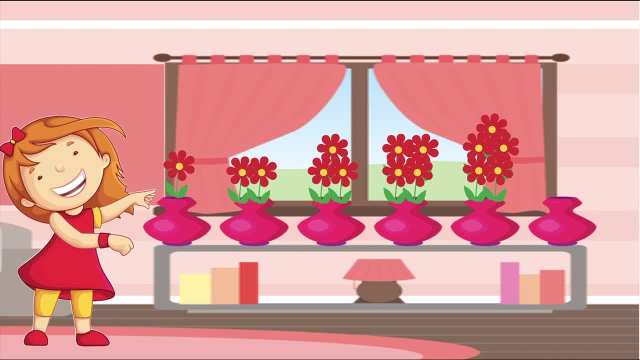 So let's count the flowers. in each vase We have 1,. on the 2nd one we have 2,, 3,, 4,, 5.. So how many flowers are there on the 6th vase? Very good children. 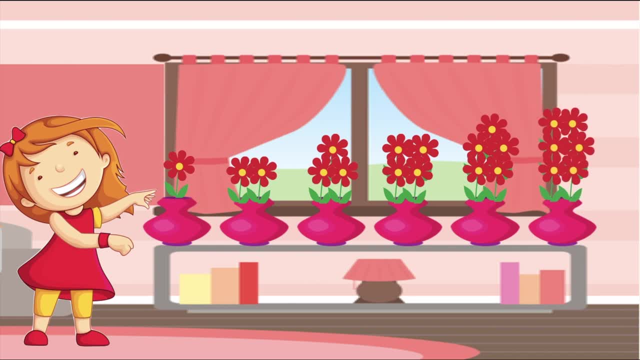 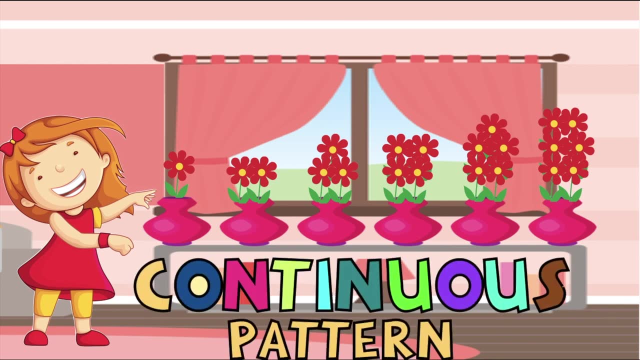 We're going to have 6 flowers. This pattern is what we called a continuous pattern. When you say continuous pattern, it is a pattern where something is added in the terms. every time the sequence repeats Again. this is what we called the continuous. 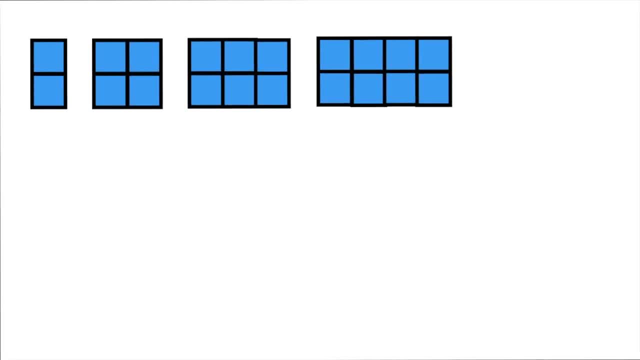 So we have a continuous pattern. How about, if I have this? So on the 1st term we have 2 boxes, on the 2nd term we have 4 boxes, on the 3rd term we have 6 boxes, and on the 4th term we have 8 boxes. 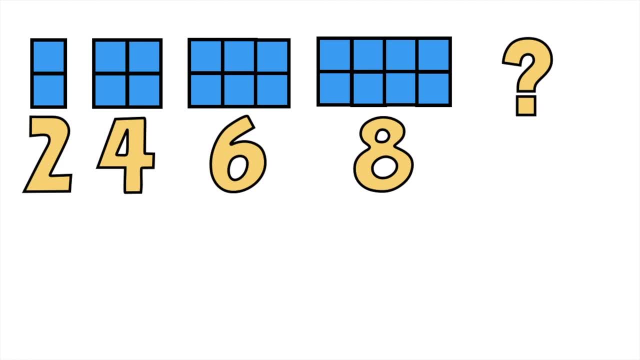 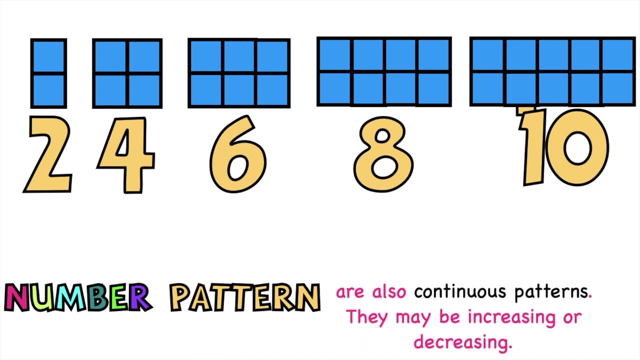 So, children, what do you think? or how many boxes do we have in the 5th term? Very good, We're going to have 10 boxes, 10 boxes, good job. This pattern is what we called the number pattern. Number patterns are also continuous patterns. 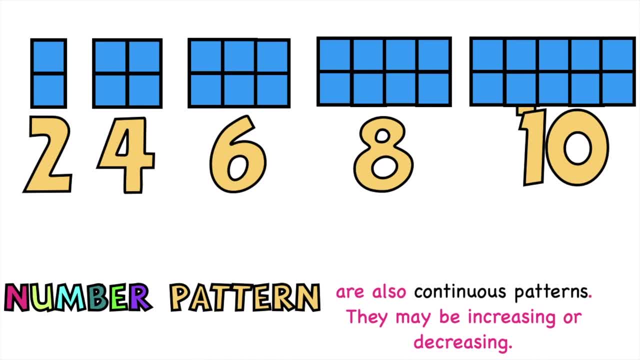 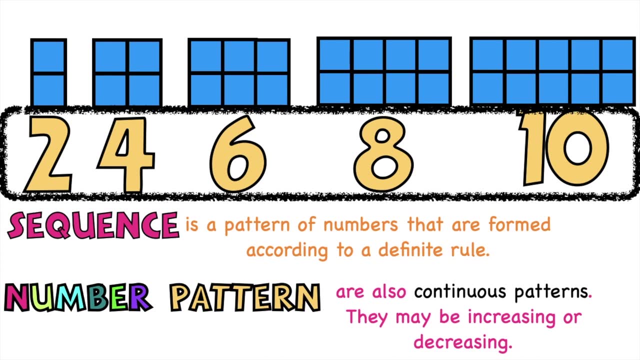 They may be increasing or decreasing Again. this is what we called the number pattern. This- 1,, 2,, 4,, 6,, 8, and 10- is what we called sequence. Sequence is a pattern of numbers that are formed according to a definite rule. 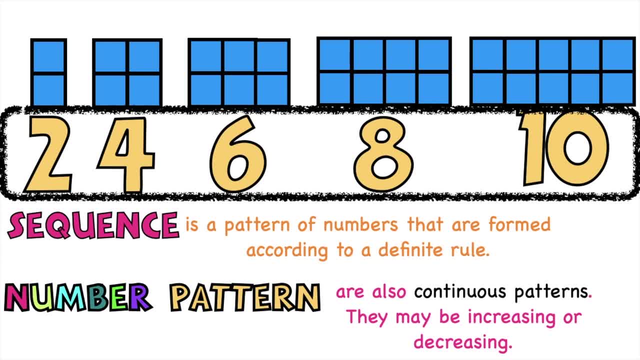 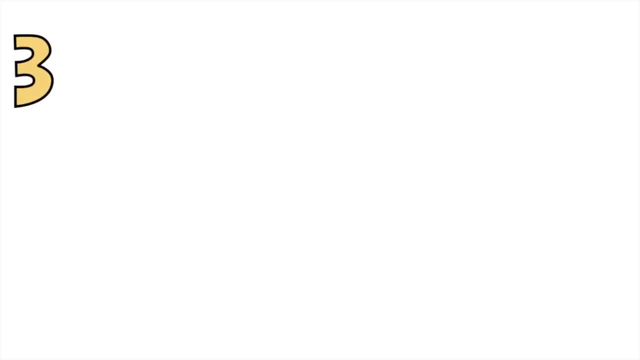 So again, this is a sequence, Is that clear? So how about if we have this: 3,, 5,, 7,, 9,, 11, 13.. What do you think will be the next 2 terms? In able to find the next 2 terms, we need to identify first the order of the numbers. 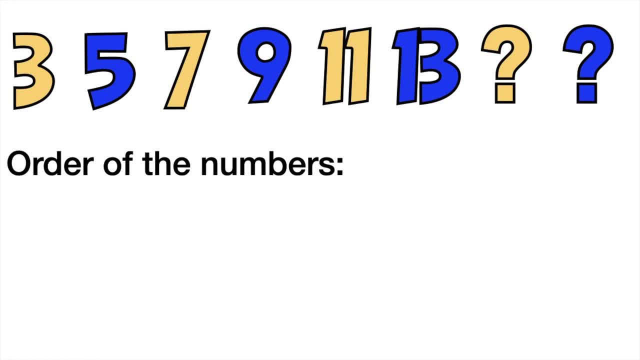 What do you think will be the next 2 terms? What do you think will be the next 2 terms? What do you think will be the next 2 terms? What do you think is the order of the numbers? Is it increasing or decreasing? 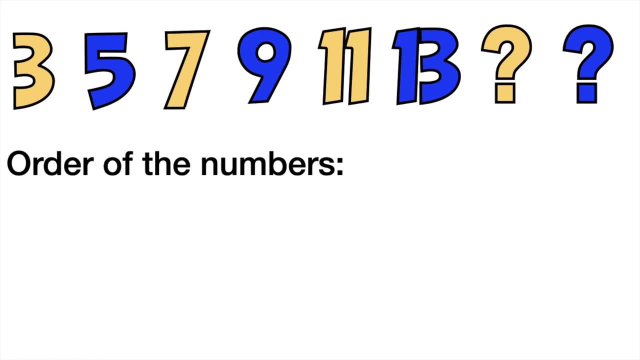 That's correct, children. The sequence is in increasing order. Next, let's find out the difference between 2 consecutive numbers. When you say 2 consecutive terms, it's the numbers that are next to each other. Okay, so now let's find the difference of 3.. 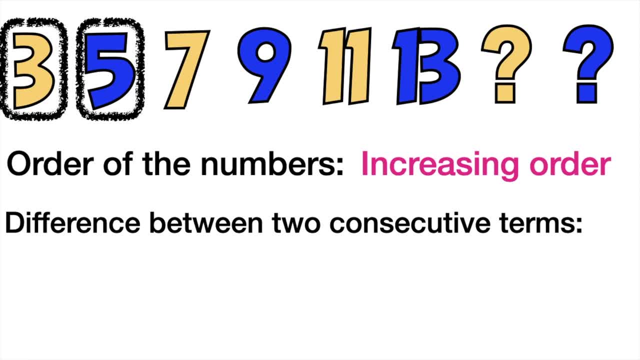 of 3 and 5. always remember children, when you are subtracting big number first, followed by a smaller number. so we have 5 minus 3 equals 2. then let's subtract 7 and 5. 7 minus 5 equals 2, very good. 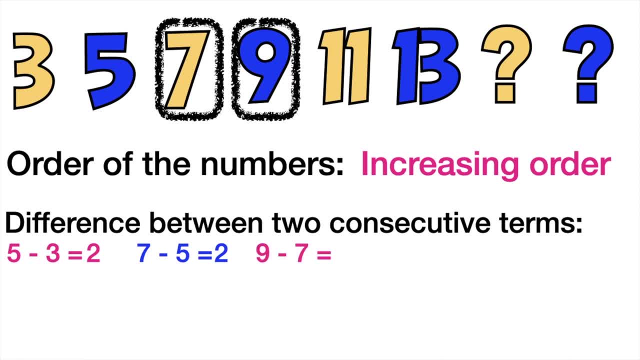 how about 9 minus 7 equals that's correct, it's 2. how about 11 minus 9 equals 2. and lastly, how about 13 minus 11 equals 2. very good, so, as you can see, the difference between two consecutive terms is always 2, so that means to find the next term. 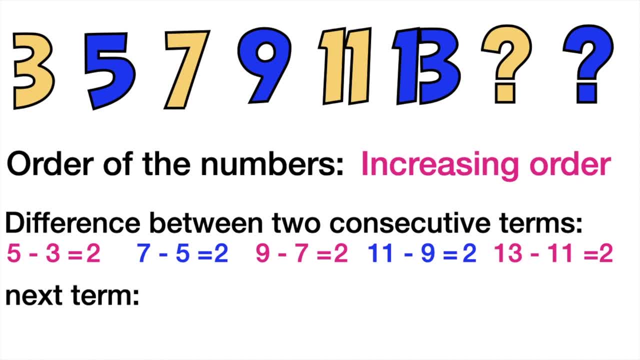 we need to subtract 7 and 5. so let's subtract 7 and 5. so let's subtract 7 and 5. so let's subtract 7 and 5. so we need to add 2 on 13, since it is increasing order. always remember children. 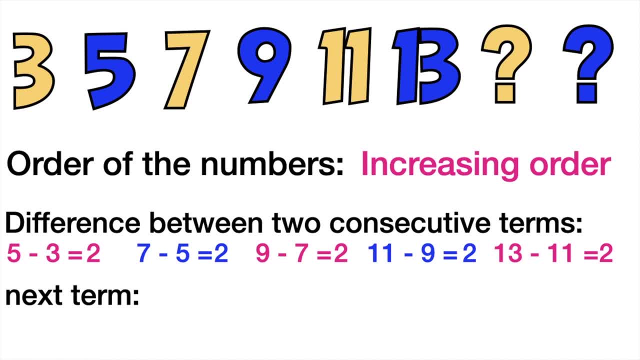 if the order of the numbers is increasing, you are going to add the difference of the two consecutive terms on the last term to find the next missing term. is that clear? so we have 13 plus 2 equals, that's correct, it's 15. so the first missing term. 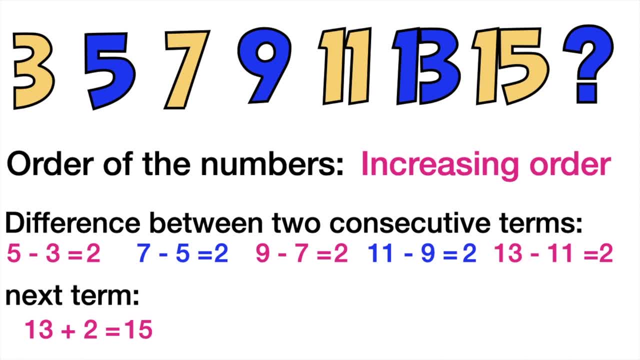 is 15. how about the next one? so we're going to add 2 to 15. 15 plus 2 equals good child genres. it's 17. so our missing terms are 15 and 17. very good. so how about if we have this? 65, 55, 45, 35, 25? so what do you think of 15? that's correct. 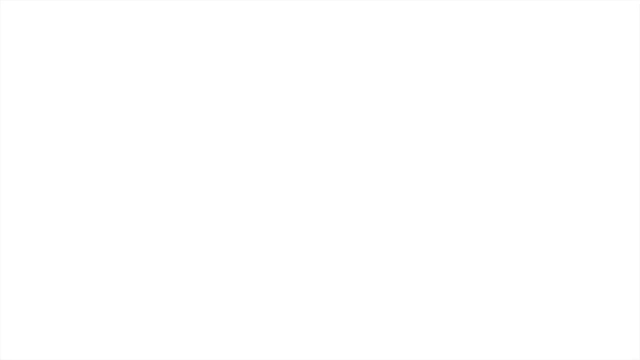 if we have 15, then we need to add 75, and arrow means 15, so that means that our numbers. What do you think are the missing terms? Again, let's find out the order of the numbers. Is it increasing or decreasing? That's correct. It's decreasing. 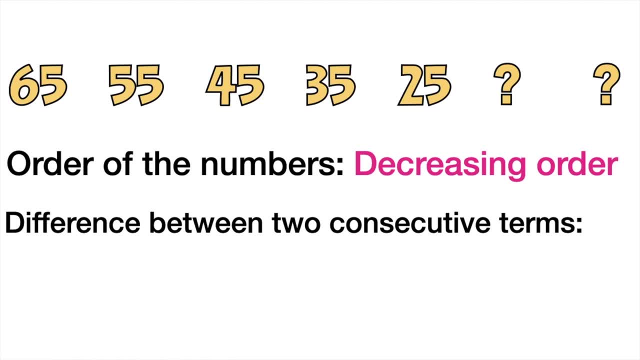 Next, let's find the difference between two consecutive terms. 65 minus 55 equals 10.. Very good. How about 55 minus 45? It's 10.. How about 45 and 35? It's also 10.. 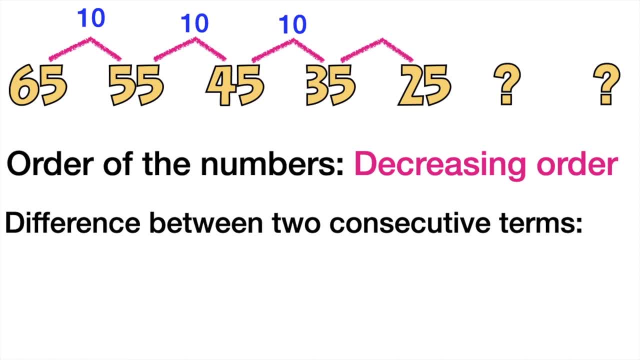 How about 35 and 25?? Good job, That is 10.. As you can see, the difference between two consecutive terms is 10.. So now let's find out the next term. Children, remember it is decreasing order, right. 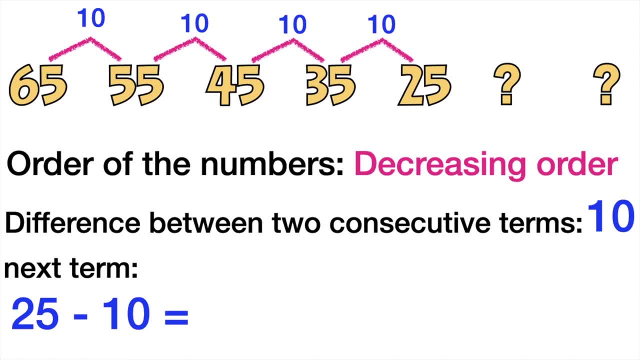 So we're going to subtract 10 to the last term, So we have 25 minus 10 equals. Very good, It's 15.. So the first missing term is 15.. How about the last missing term? We have 15 minus 10 equals. 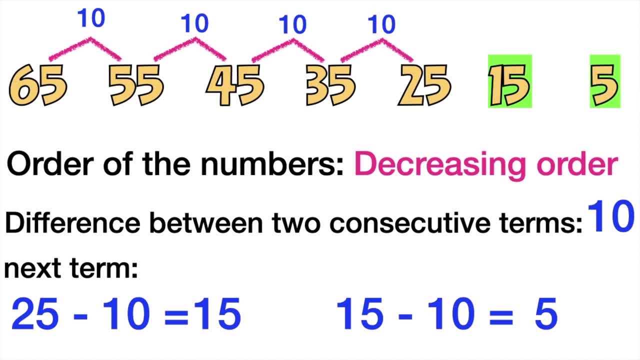 That's correct, It's 5.. So our last term is 5.. So we have 65,, 55,, 45,, 35,, 25,, 15, and 5.. That's correct. However, 5 and 5 are the same. 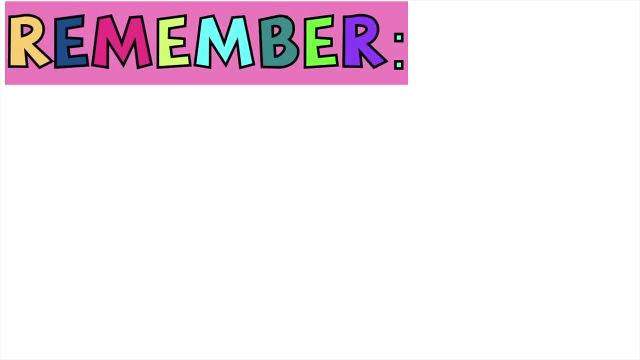 The last time we said 55.. The last time we said 5.. So that means we have 55. That's right. Now we're going to go ahead and write a new one, Our next one. It's called the large interval. 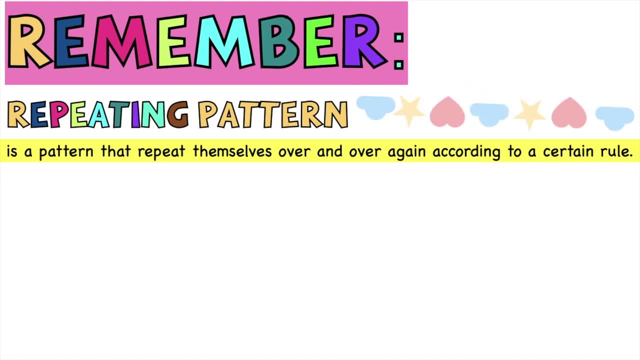 It's really easy to spell. Well, let's do the same thing. The first time, we say 55.. The second time, we say 55.. That's correct. So now we have 8, 6, 5, 6, 6, 7, 8, 1, 2, 2, 1, 2, 2, 2, 3, 2, 3, 2, 1, 2, 1, 2, 2, 4, 5.. 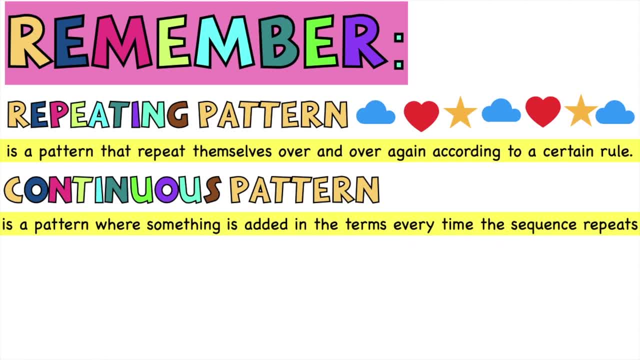 That's correct. How about 55?? That's correct. a pattern where something is added in the terms. every time the sequence repeats. for example, we have this: as you can see, the circle becomes bigger and bigger and bigger. and the last one: we also have what we call the number pattern. number pattern are also continuous patterns. they may 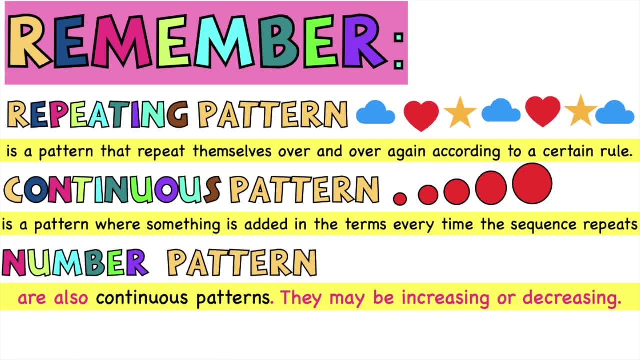 be increasing or decreasing. always remember, children, how to find the next term in the number pattern. the first thing that you need to do is to find the difference between the two consecutive terms. then if it is increasing, you're gonna add, but if it is decreasing you're going to. 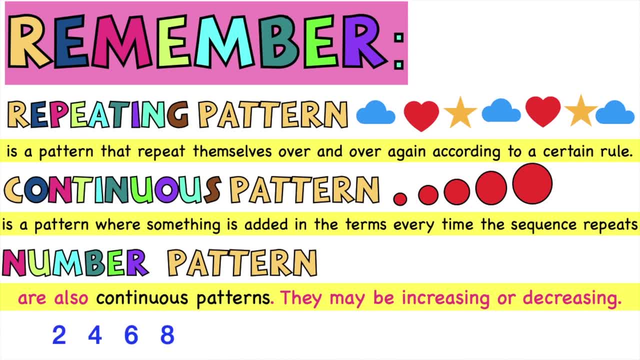 subtract. for example, we have 2, 4, 6, 8- this is increasing pattern- and 27, 27, 27, 24,, 21,, 18.. This is decreasing, Is that clear? So now it's your turn. Get your drill board. 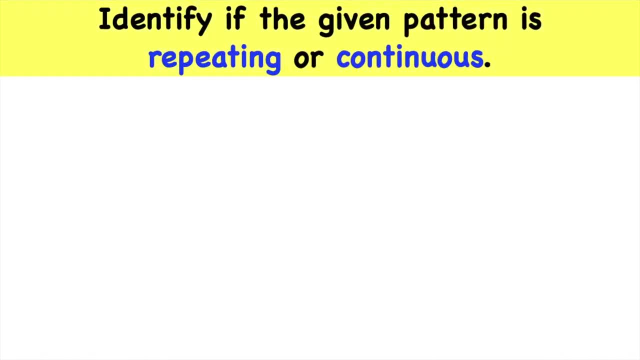 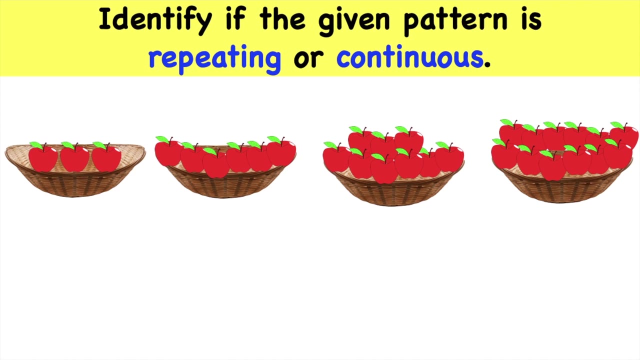 Using your drill board, I want you to identify if the given pattern is repeating or continuous. Are you ready? Let's have the first one. Is it repeating or continuous? The correct answer is continuous pattern Because, as you can see, the numbers of apples become bigger and bigger. 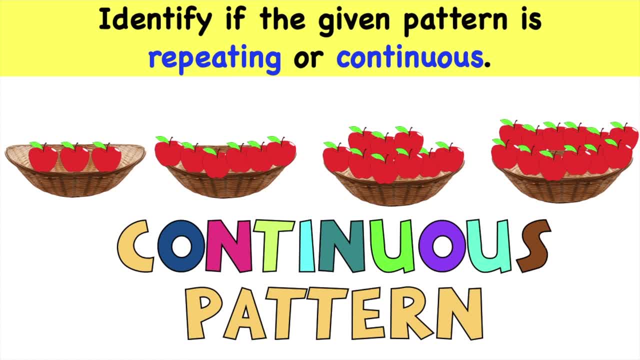 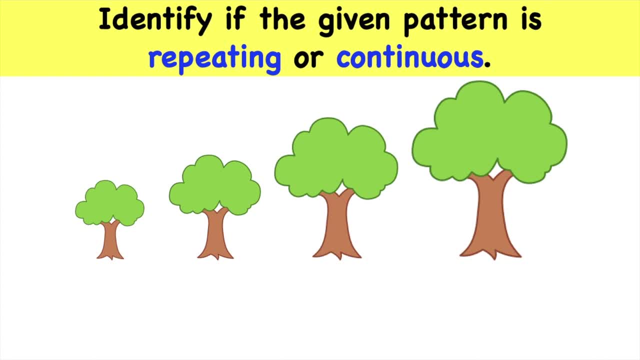 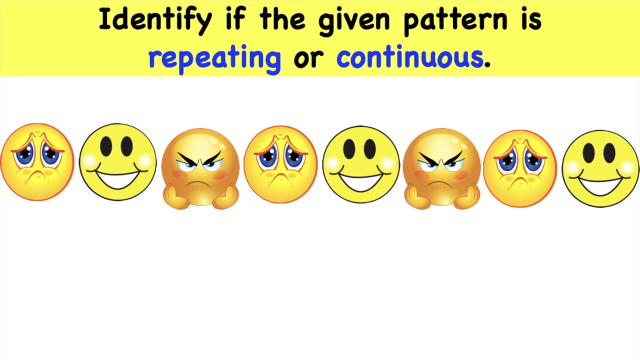 That's why it is a continuous pattern. How about if we have this? Is it repeating or continuous? That's correct, children, It is a continuous pattern. How about if we have this? Is it repeating or continuous? Very good, It is a repeating pattern. 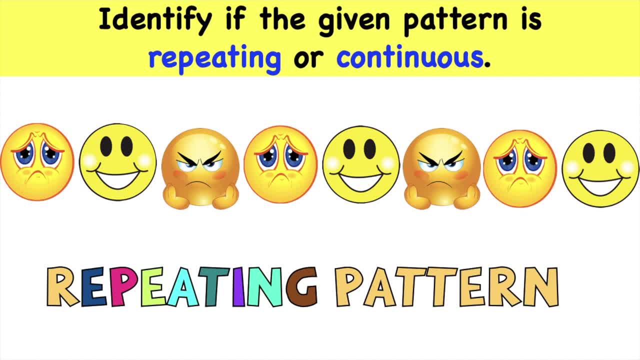 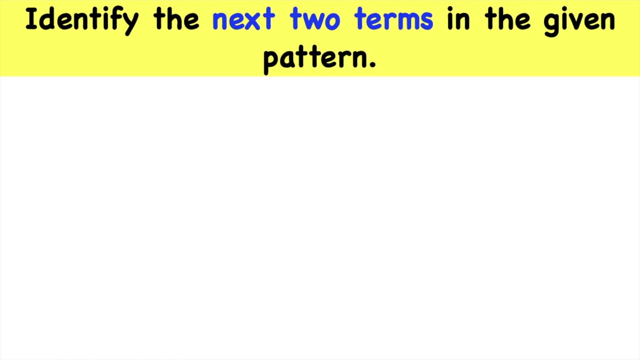 Because, as you can see, the terms are sad, happy, angry, sad, Happy, Happy, angry, sad, happy. That is a repeating pattern. So now let's identify the next two terms in the given pattern. Are you ready, kids? 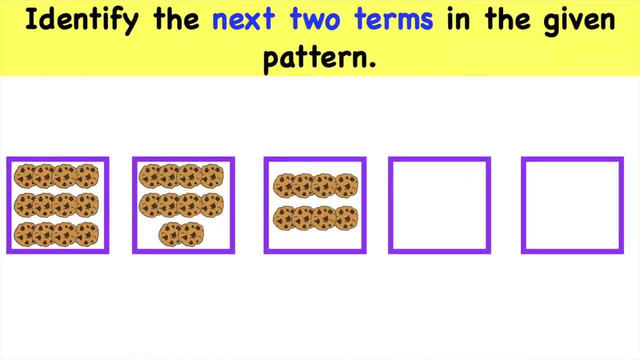 So let's have the first one. What do you think is the missing term? So let's see if your answer is correct. The first missing term is six cookies And the last term is four cookies. Very good children, We have twelve, ten, eight, six, four. 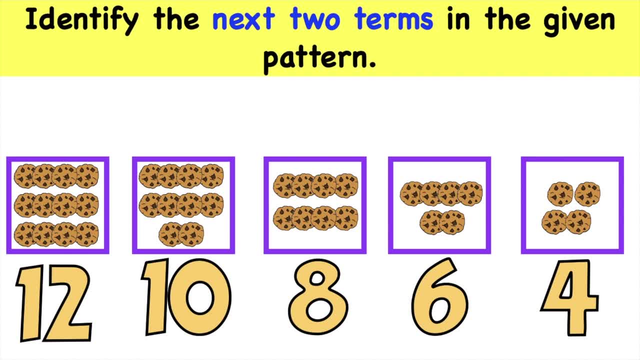 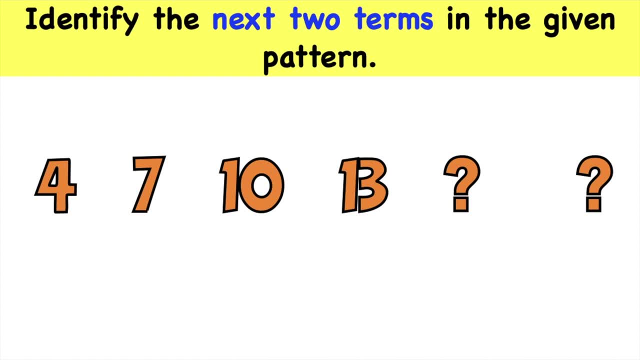 So this is a continuous pattern, right? How about if we have this Four, seven, ten, thirteen, blank, blank? What do you think? What do you think are the next two terms? Let's find out if your answer is correct. 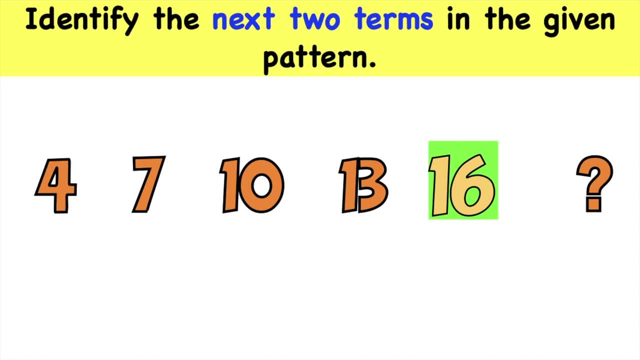 The first missing term is sixteen And the last missing term is nineteen. Always remember children how to find the missing terms in a number pattern. The first thing that you need to do is to find the difference of the two consecutive terms. We have seven minus four equals three. 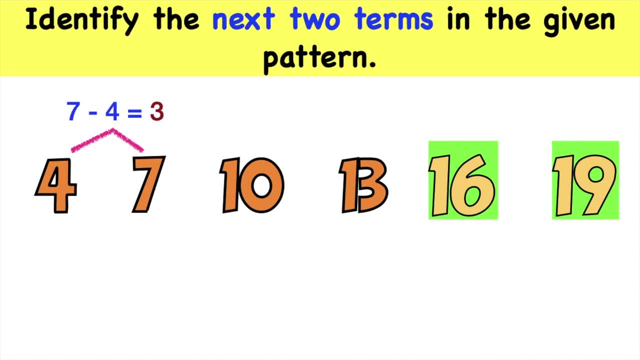 Then all you need to do, since the sequence is in increasing order- you're going to add three to the last term, which is thirteen. Thirteen plus three equals sixteen. Then add three to sixteen. Sixteen plus three equals nineteen.